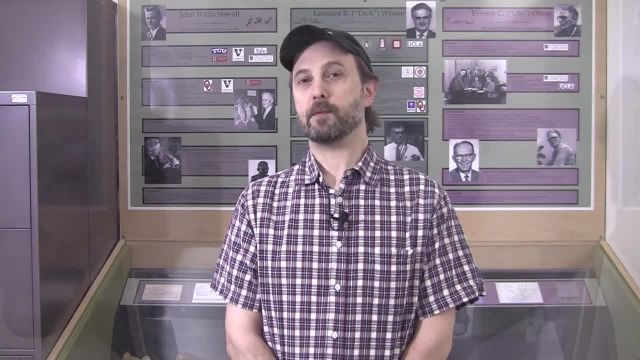 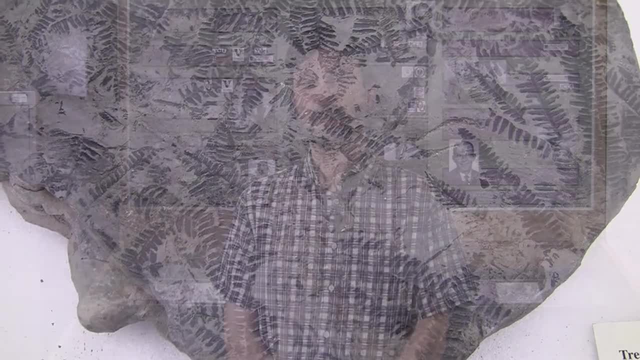 about my science of paleobotany is when you split open rocks and you finally see plants, the remains of plants that no human has ever seen before. It's a form of time travel and it's cool to think about the way things used to be and the plants and the animals that 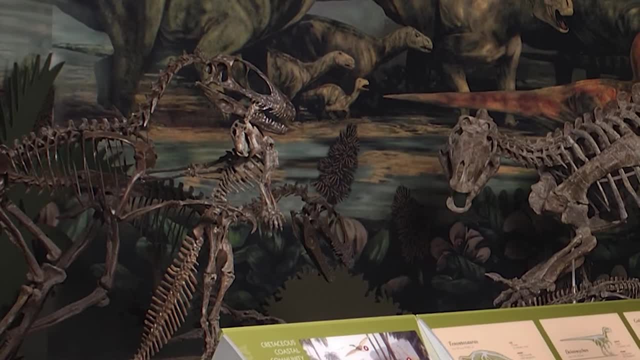 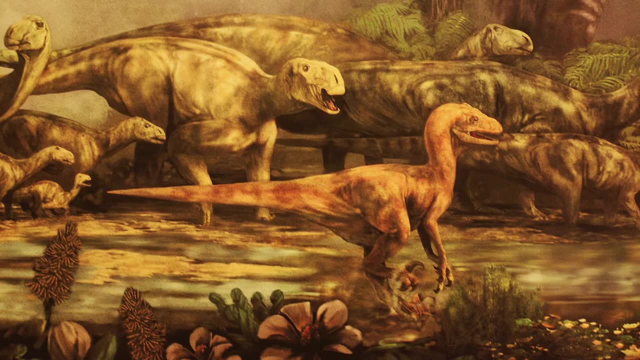 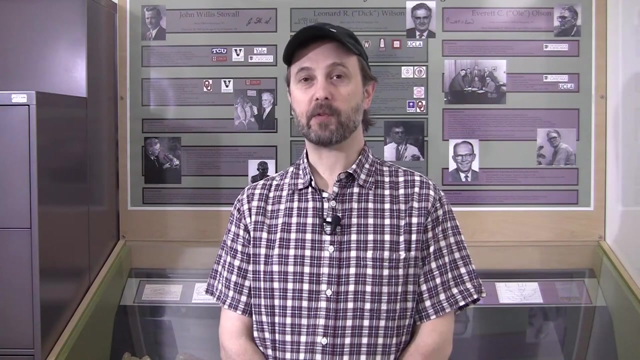 used to live on earth. Dinosaur fossils and the fossils of other animals are cool, but there's so much more that we can learn. Fossils of plants tell us about what those dinosaurs did, the nature of the habitat in which they lived. So when we ask questions about modern 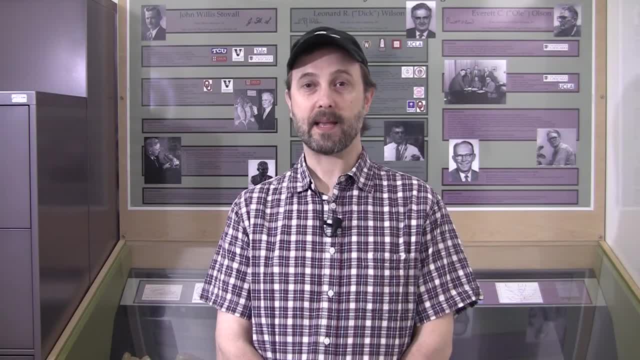 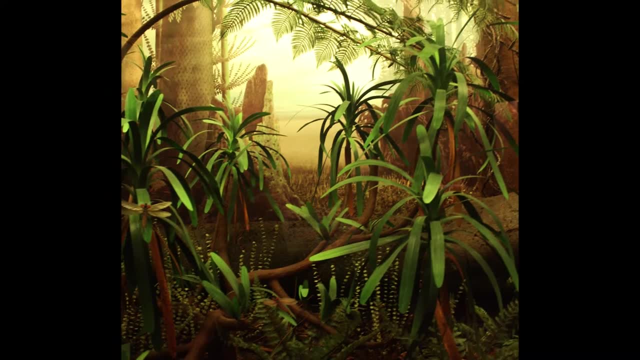 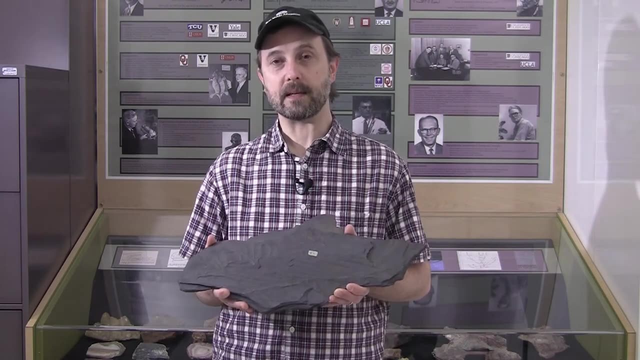 climate change. plant fossils give us an important context, a background with which you understand how animals and plants and life on earth have changed over time. One of the most interesting objects in our collection is this plant fossil from Rhode Island. This rock preserves the 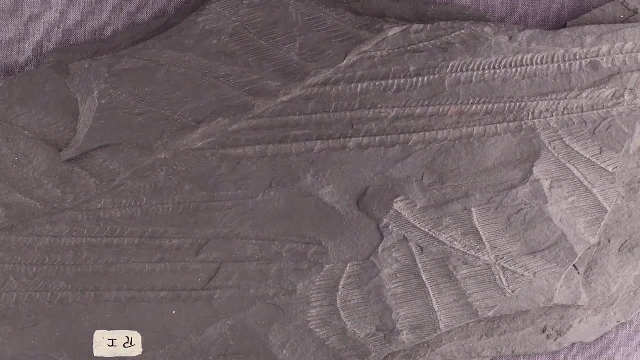 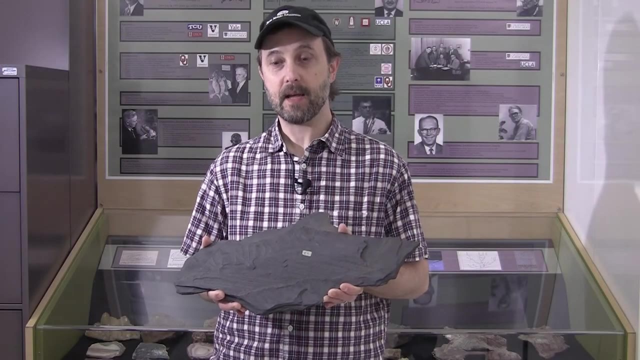 remains of a fern that were buried in sediment about 300 million years ago. This rock is one of the most important objects in our collection. When North American Africa collided to form the supercontinent of Pangea, it stretched these rocks By measuring the plants on this. 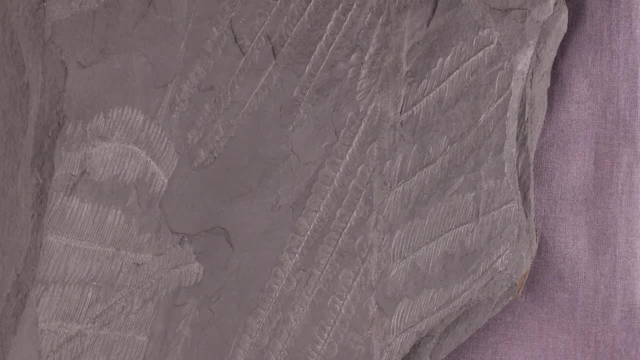 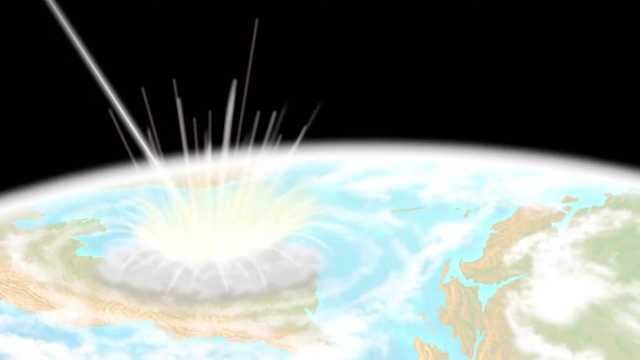 rock. we can see that the rock was stretched about three times its original size as part of that collision. When a rock or piece of iron traveling through space enters earth's atmosphere, we call it a meteor If it strikes the ground and there's debris left to be found. 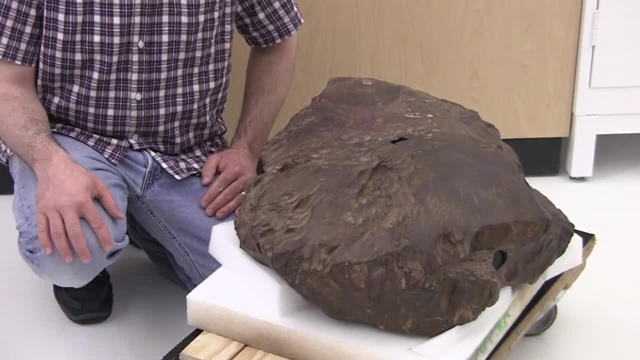 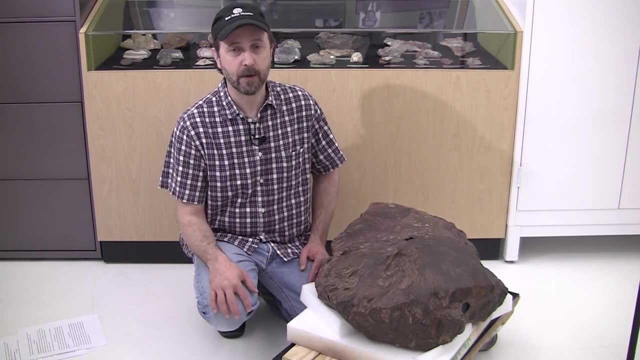 we call it a meteorite. This is the Keys meteorite. This meteorite is a meteorite that has been found in the state of Oklahoma. This is named for the town in Oklahoma near which it fell At 142 kilograms, or about the size of a good football linebacker. this is one of the largest. 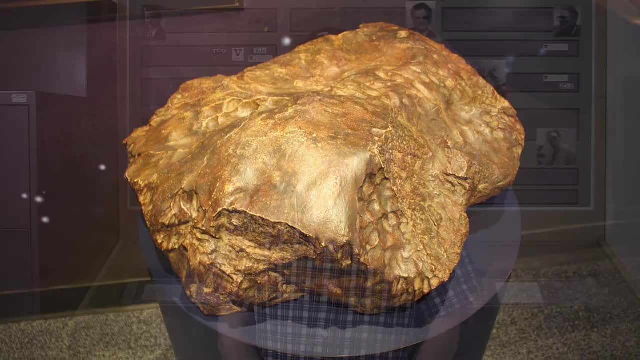 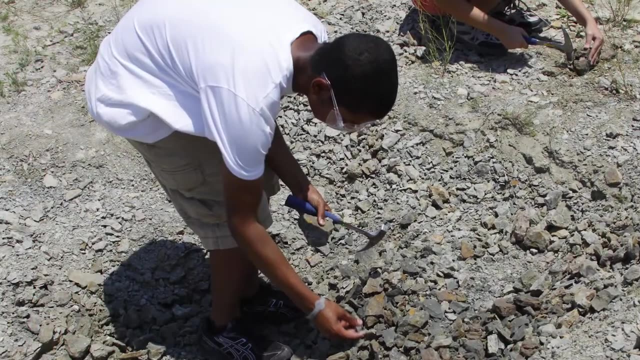 meteorites ever found in the state of Oklahoma. You should be interested in science, even make a career out of it, if you're curious about the world around you. We need more scientists. Scientists are the ones who discover cures for diseases, work out new crops and ways. 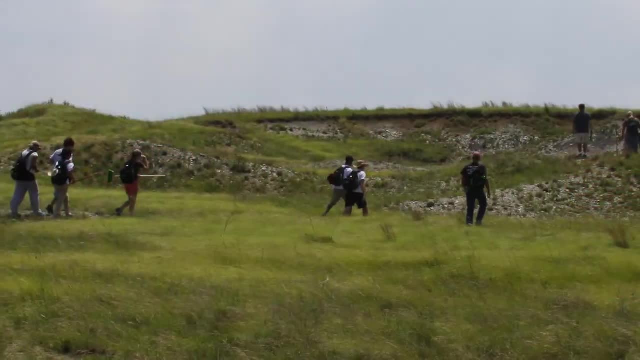 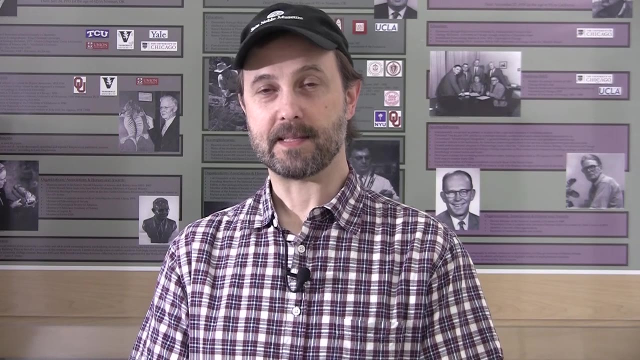 to feed people, And science is the opportunity, provides the opportunity to explore the world. Explore, learn and serve. Thank you for joining me in the Paleobotany collection at the Sam Noble Oklahoma Museum of Natural History.